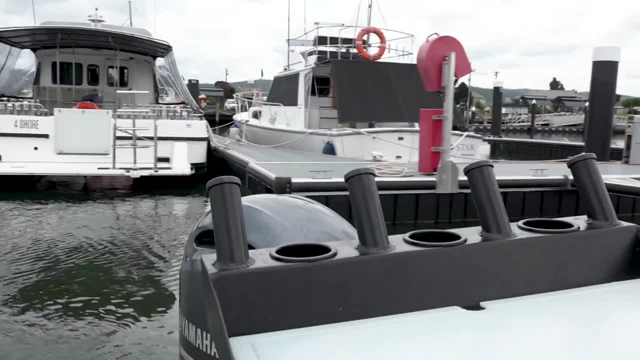 spaces. it can cause problems because the back of the boat will move in the opposite direction to where it's supposed to go. So if you've got a boat that's got a lot of power and a lot of power, you want the front to go. This can be unhelpful. Don't be afraid to use a reverse. 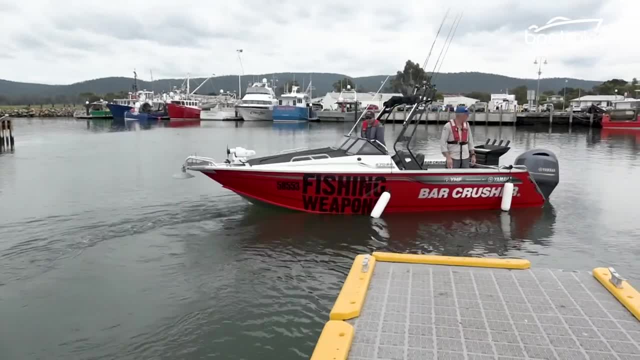 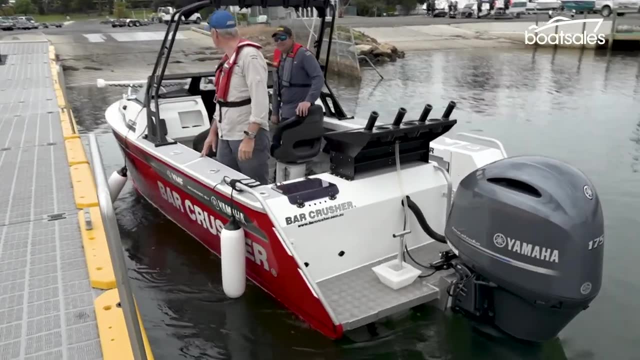 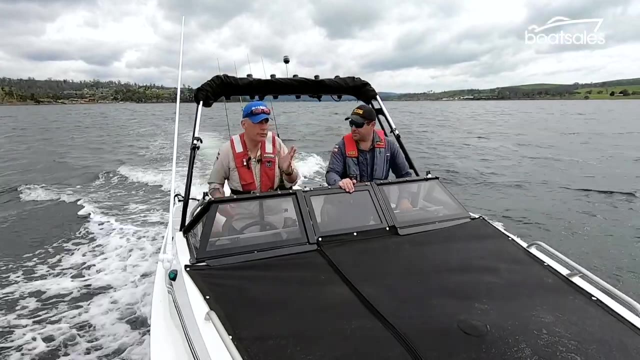 gear, The stern will go where you point it and the bow will generally follow. Remember, if you need to get out of a tight spot, backwards is your friend. Probably one of the most technical aspects of driving a boat, Andrew, is the notion of trim, where your outboard is in relation to 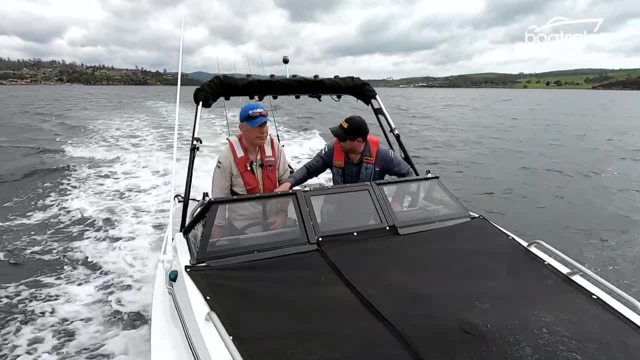 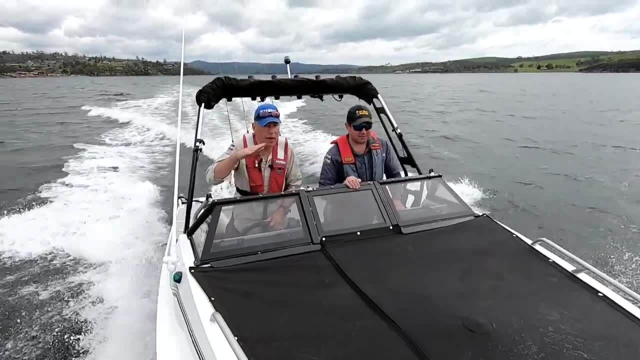 your transom, Nick. you control it with a little button on your throttle- up and down, up and down- and it's about finding the right place. When you take off, typically you'll have your engine trimmed all the way in and that will allow your boat to come up onto the plane. 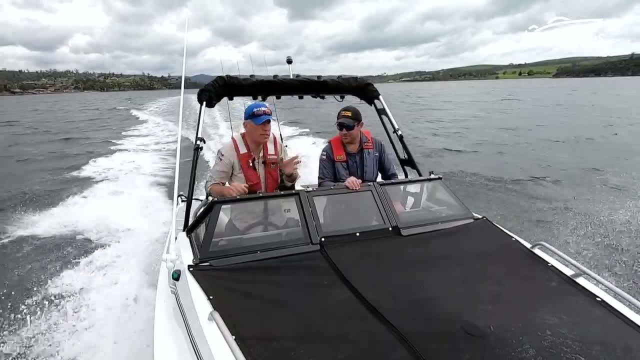 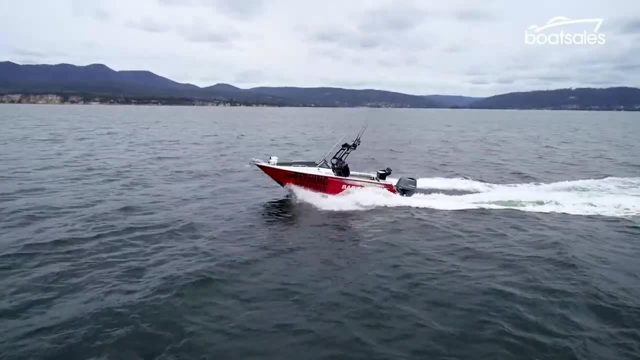 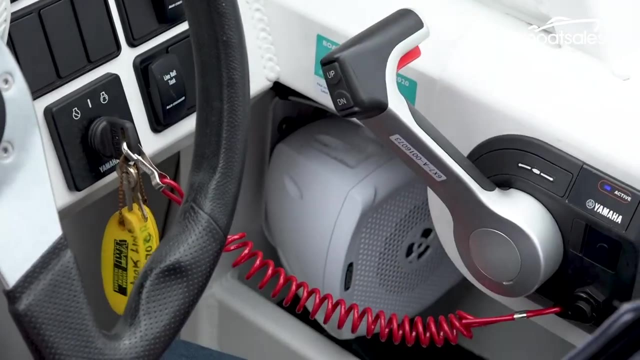 nice and flat. Then it's about deciding what sort of trim state suits the water you're travelling across. The simple rule of thumb is: trim in when heading into the waves. That keeps the bow down and the sharpest part of the hull to carve your path. Conversely, trim up, heading with the sea. 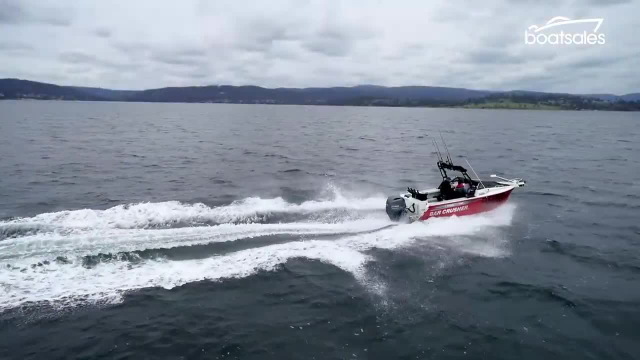 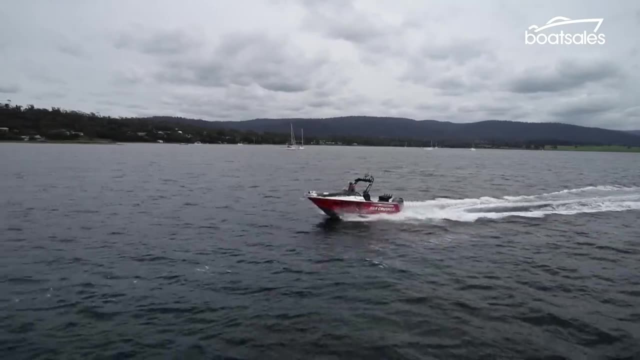 gets the bow up and the hull surfing down the back A bit of up. trim in calm water makes steering lighter and improves fuel economy. The important thing about trim is to use it. A properly trimmed boat will run rings around one that's out of whack. 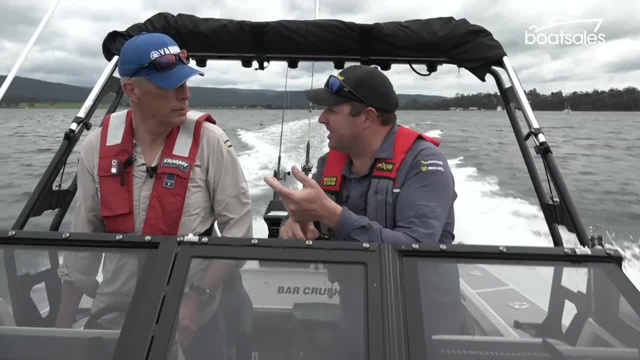 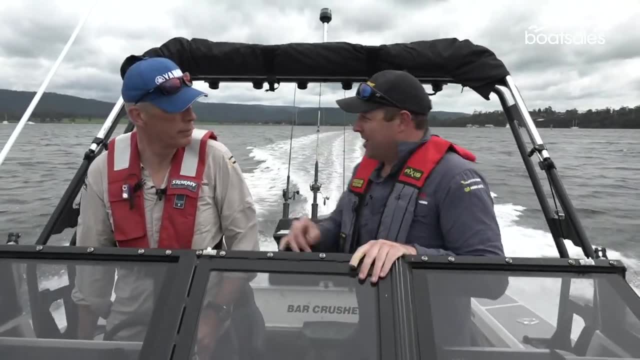 Give some thought about the load on your boat. I'm talking about eskies, maybe fuel tanks or batteries. You want everything nice and even More to the point, you want your passengers nice and even Watch this. Oh no, that's no good. We're on the point of. 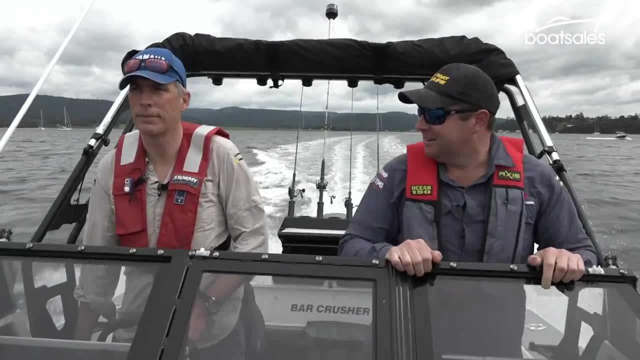 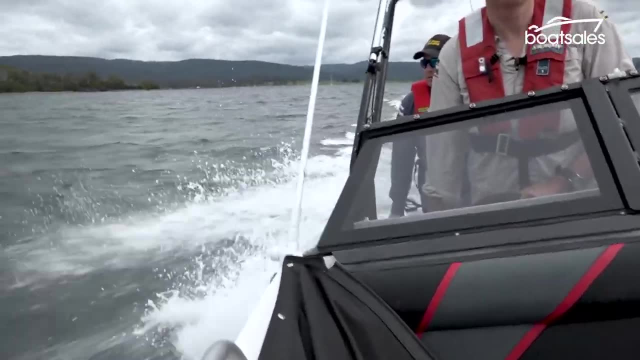 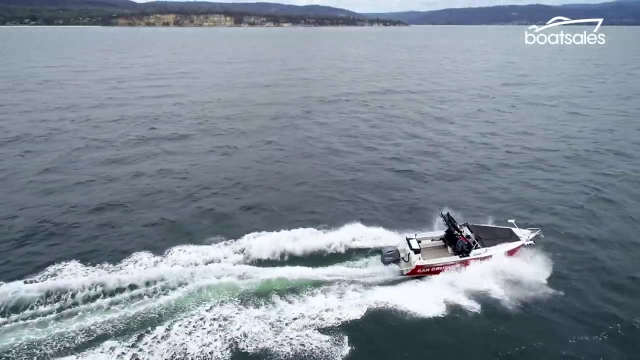 size. I'm not happy. Nothing ruins a boat's ride like having it lay over on its side. Clever hull design is immediately undone as the flat sections slam against waves. Adjust the load of people and things to keep the boat on an even keel. Boats also have the habit of leaning over into the wind. 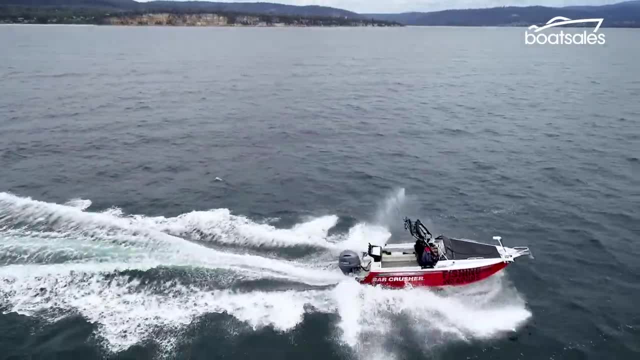 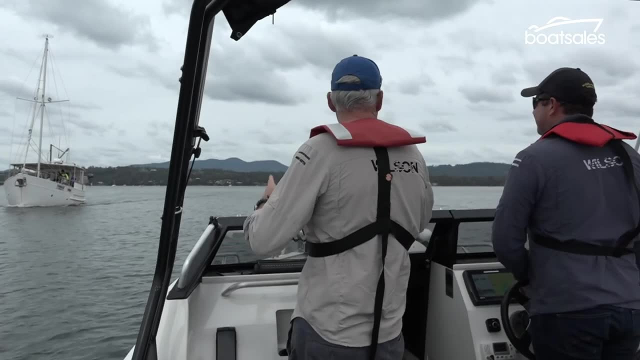 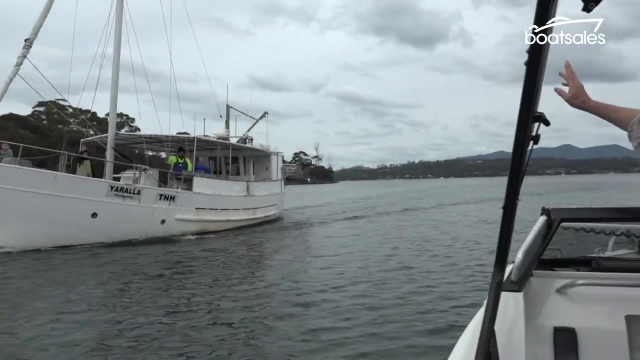 so your load arrangement may need to change as conditions do. There are also rules of the road that you need to get your head around- The difference between red and green, Andrew- and it's important that everybody can do it intuitively so as we're all on the same page, because the last